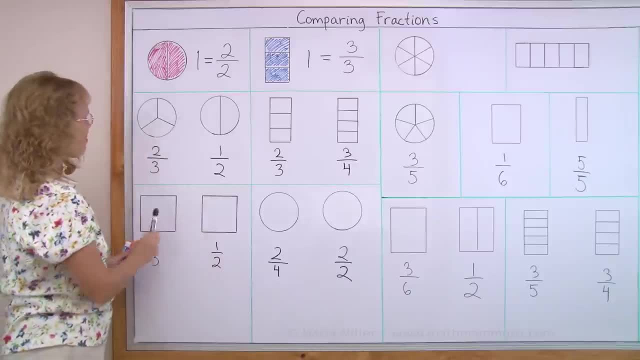 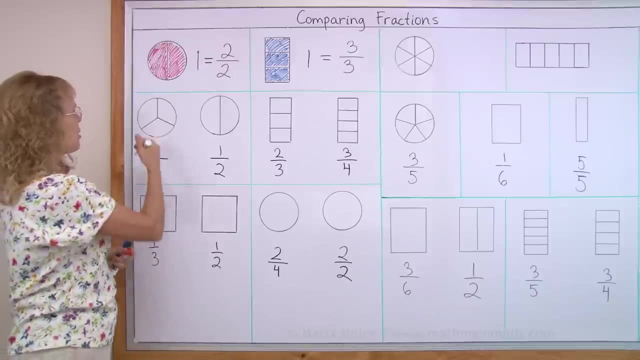 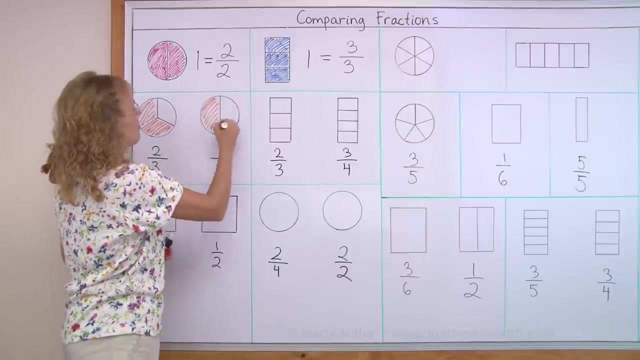 of fun because you get to color. Okay, what fraction is this? Two thirds, And that means I would color two of these parts here And over. here we have one half, so I color one part And now we compare which is greater. 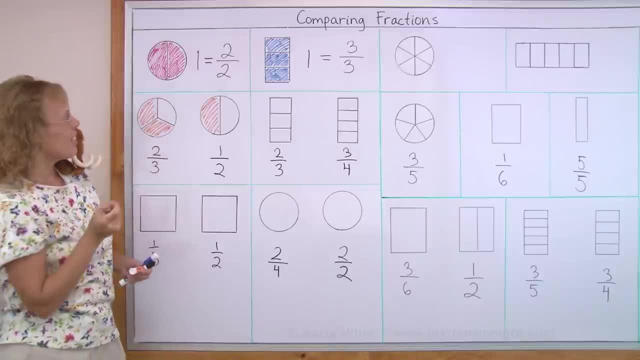 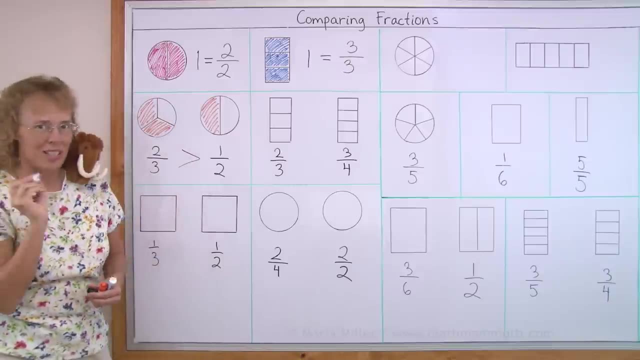 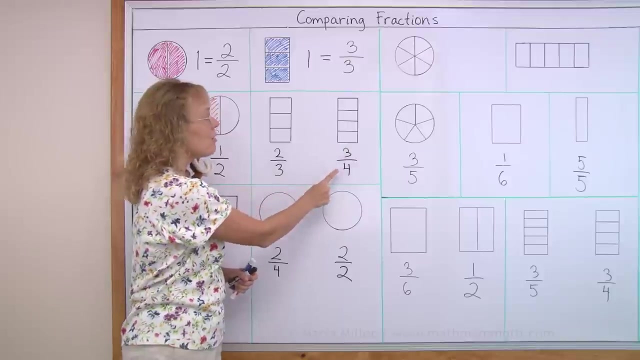 Which is more pie to eat, so to speak. You can think of it as a pie, you know, And so you see. oh, this is more right. So the alligator mouth goes that way Over here. two thirds, and what fraction is this? Three fourths, So I need to color again. Two thirds. 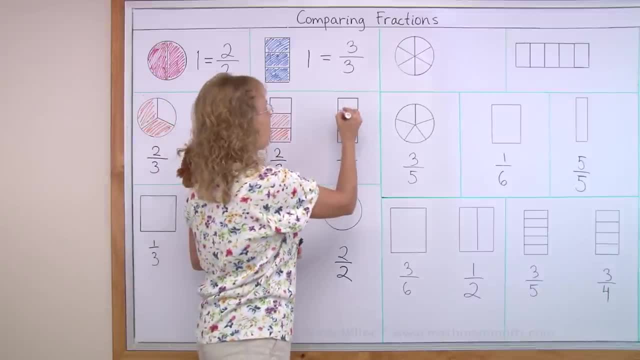 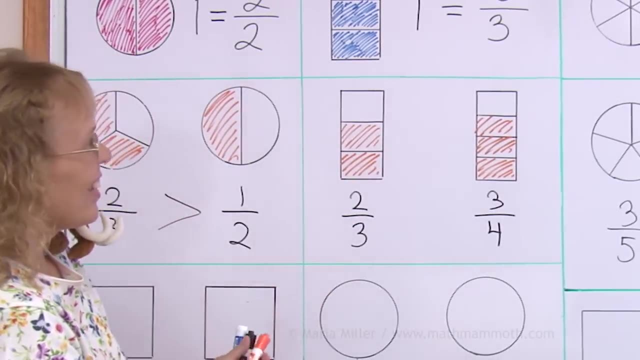 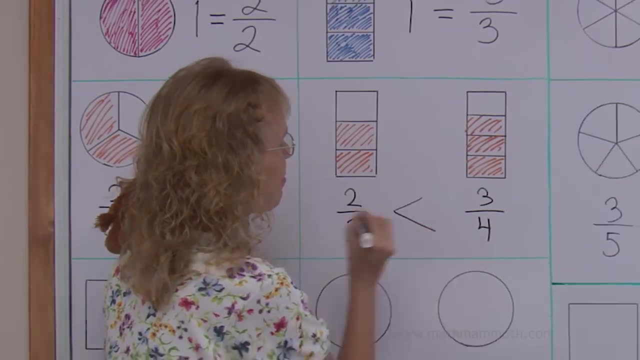 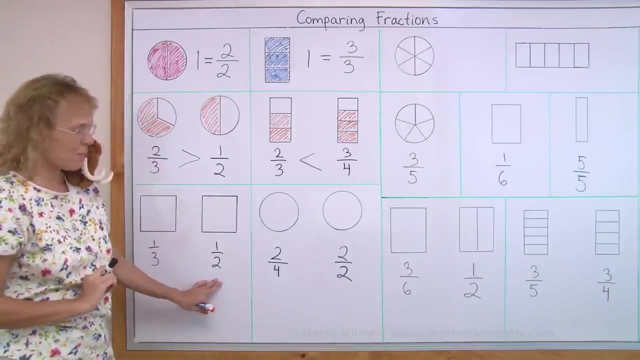 and three fourths. And which one is more? chocolate bar to eat. You can see, over here this one is a little higher, so that's the greater fraction. Over here we compare one third, one half. You want to guess which one will be the greater fraction? And once you 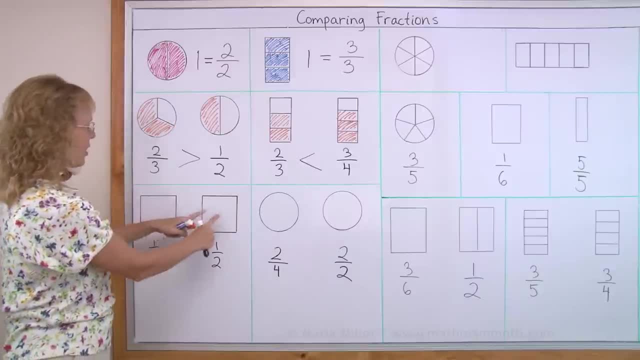 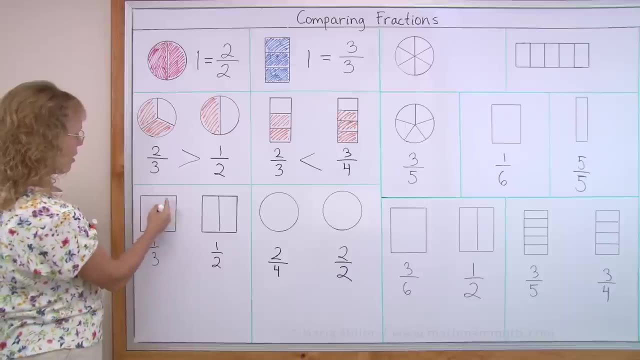 have your guess. now I'm going to have to divide this here into three quarters. So we do three parts and this here into two parts, Like that, And then this one. I could divide it this way or this way, But can you see which one will be easier way, so we can. 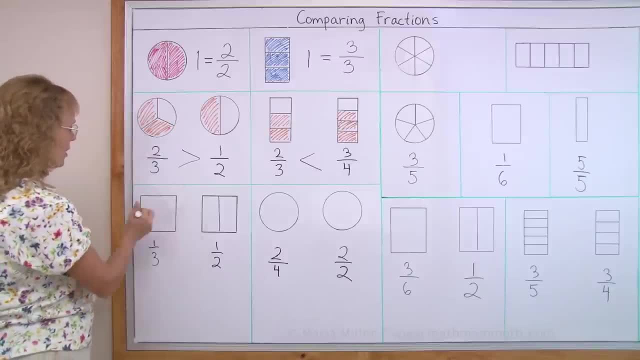 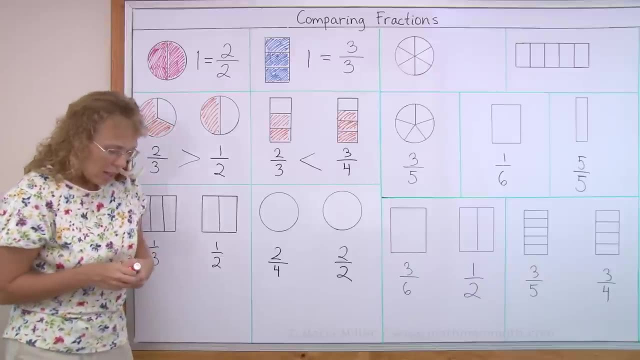 compare. If I divide it this way, it might not be as easy, so I'll divide it kind of the same way with vertical lines. Now it's time to color. Okay, Matthew. okay, I'll let you color. He's anxious to color too. Sure enough. One third, yeah, And then I'm going. 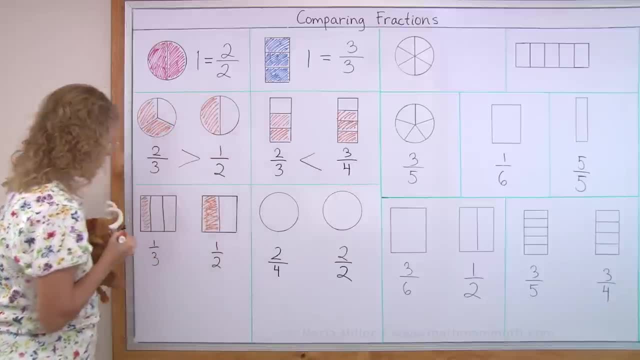 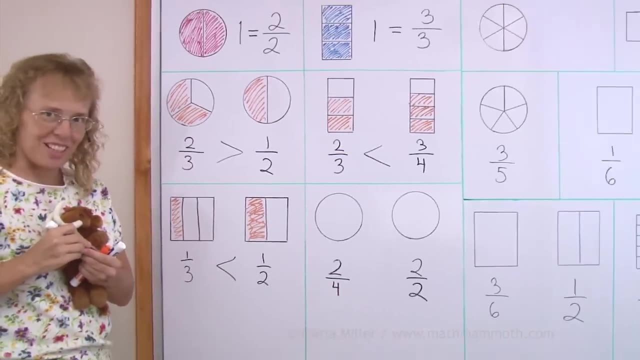 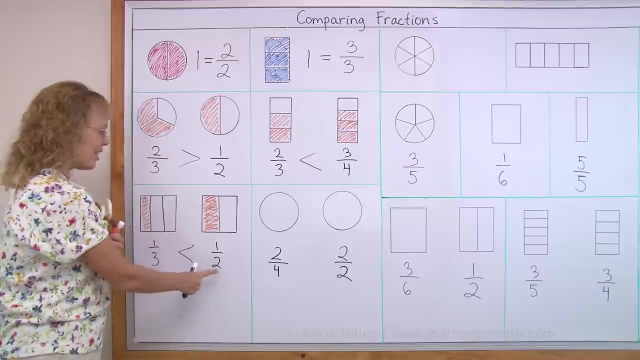 over here. one half Color, one half, Matthew. Good job. Now, which one is more? This one, of course, So one half is the greater fraction. Notice, though, that this number two is actually the smaller number than the number three, But it actually tells us into how many parts. 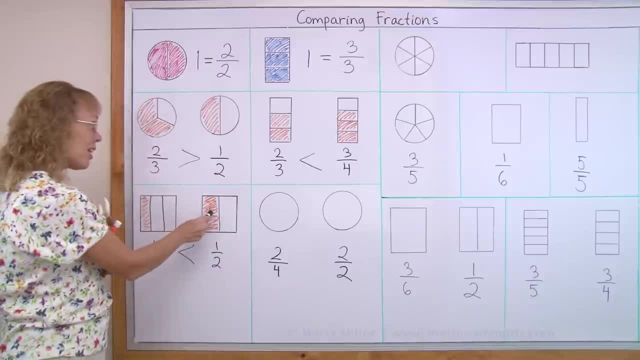 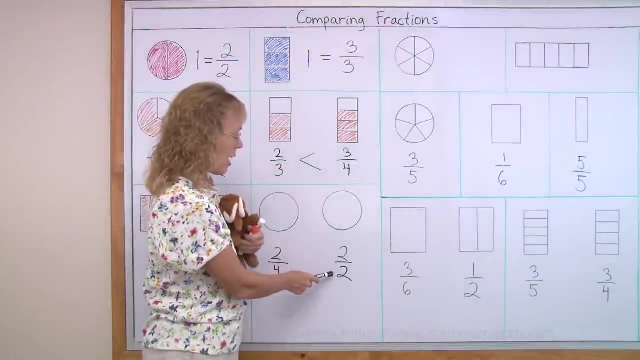 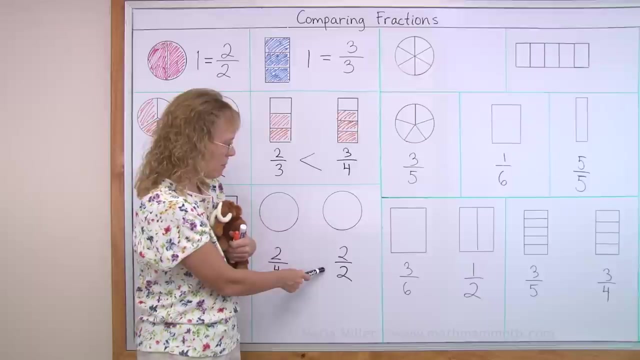 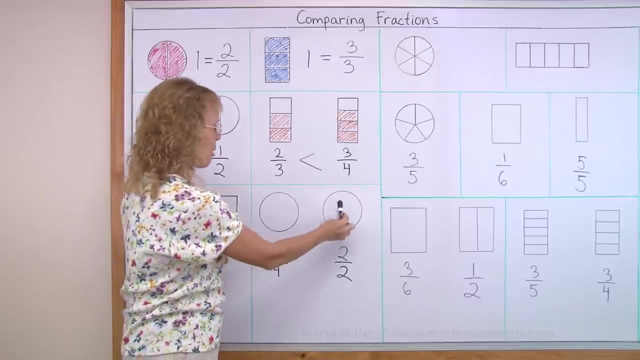 we are dividing our shape, And so this one half is still. it's more to eat than this. Two fourths And two halves. Look at this. Have we seen something like this in this lesson already Over here? Two halves is the same as the whole pie, isn't it? So I would color the whole. 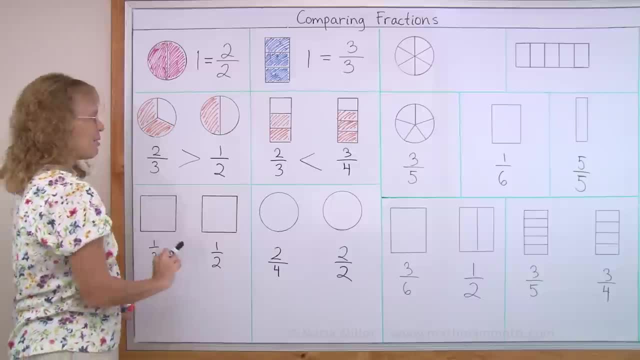 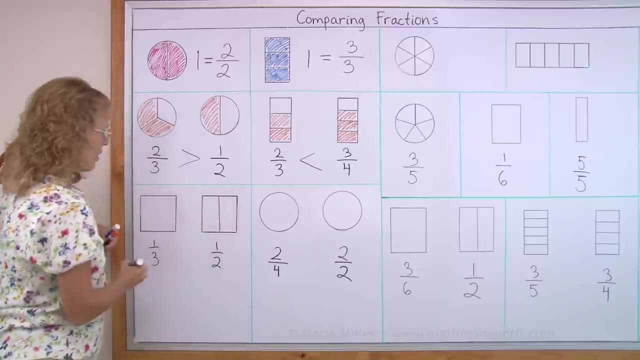 fraction, And once you have your guess now, I'm going to have to divide this here Into three parts and this here into two parts, Like that, And then this one. I could divide it this way or this way, But can you see? 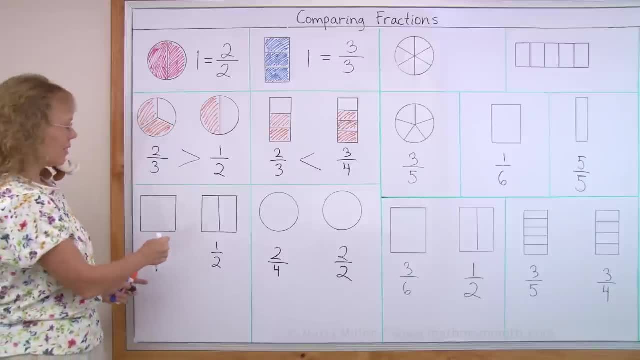 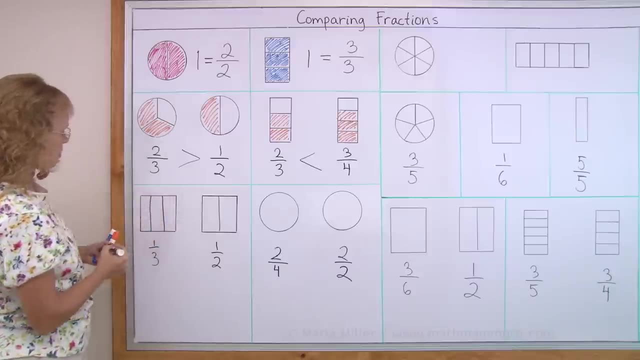 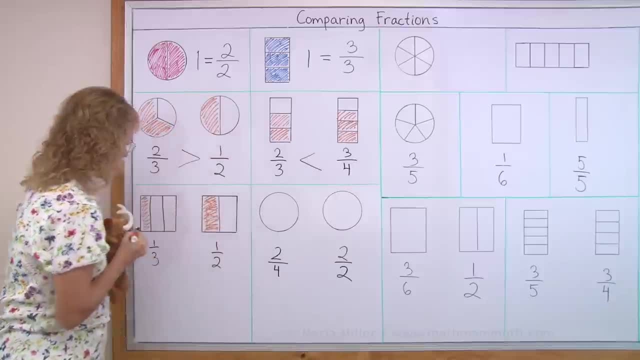 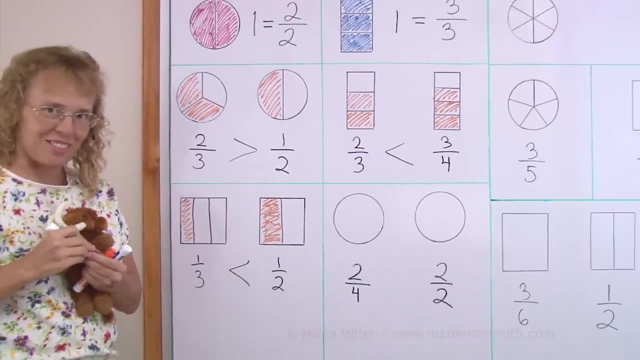 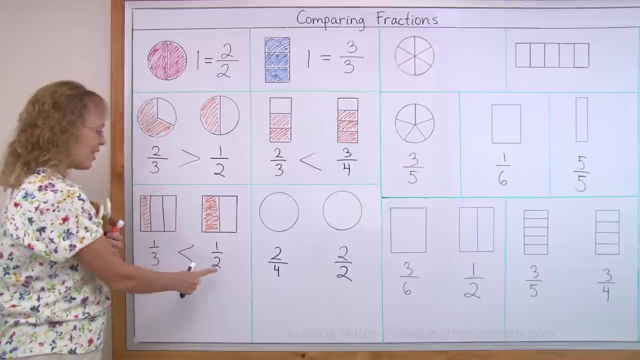 And then over here, one half Color, one half, Matthew. Good job, Now, which one is more? This one, of course, so one half is the greater fraction. Notice, though, that this number two is actually a smaller number than the number three, But 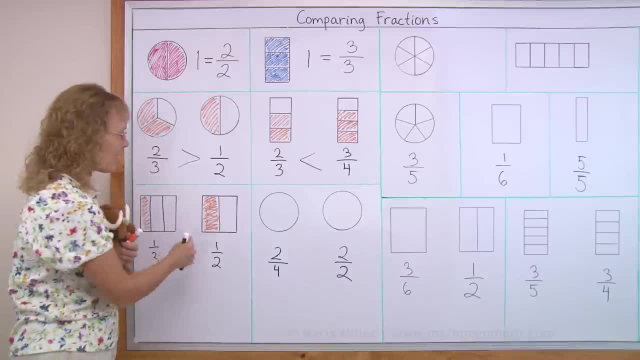 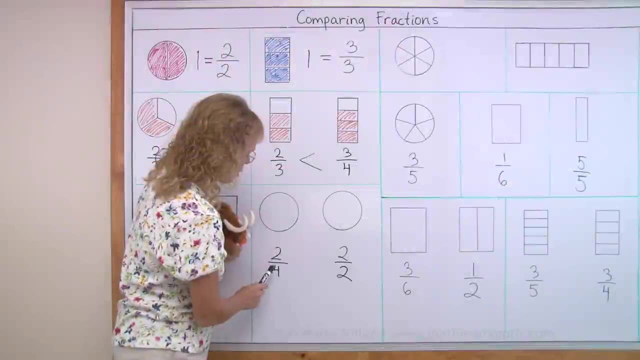 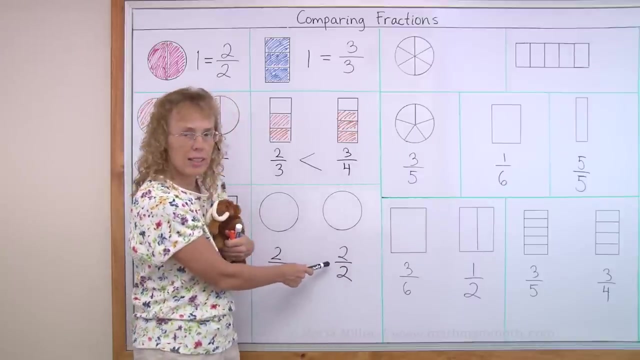 it actually tells us into how many parts we are dividing our shape, And so this one half is still—it's more to eat than this. Two-fourths Okay, and two halves. Look at this. Have we seen something like this in this lesson already? 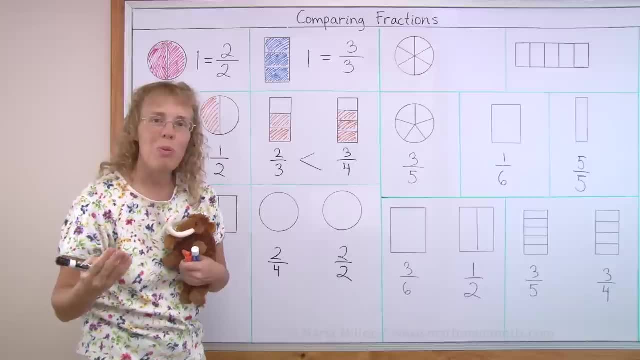 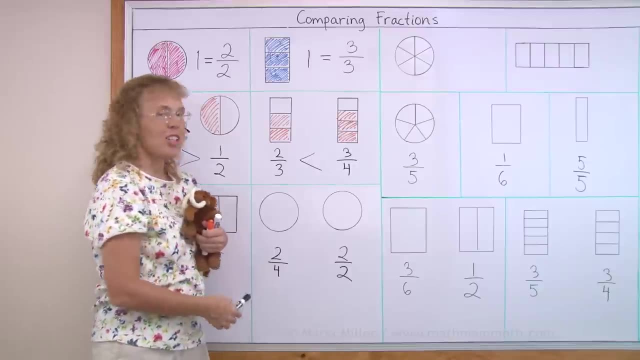 Over here. Two halves is the same as the whole pie, isn't it? So I would color the whole pie Here. I won't color the whole pie, So I can save some time and just tell that this is the greater fraction, right? 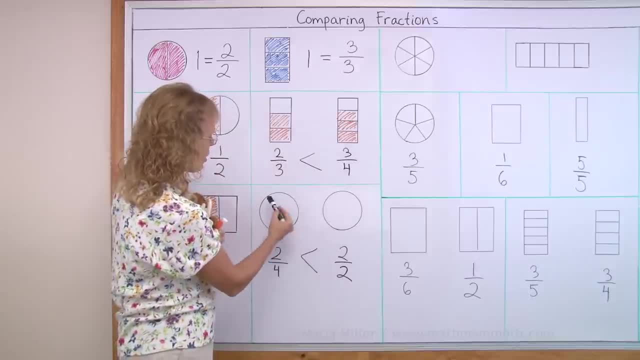 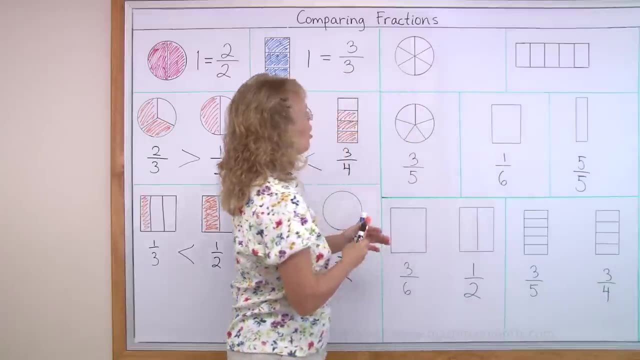 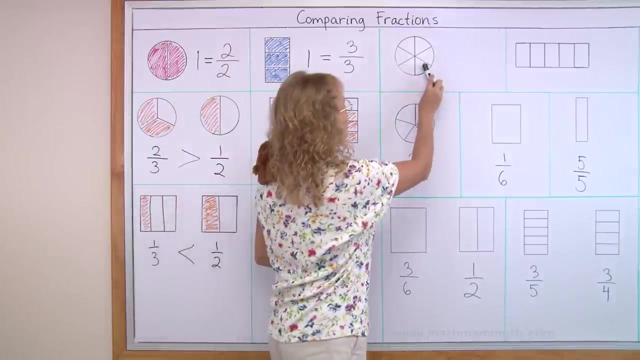 That's the whole pie. This would be if I divide it into fourths and then color two. Let's go on Over here. Well, Matti, go back here. How many parts is this pie? divided into Six parts? So each part is a sixth. 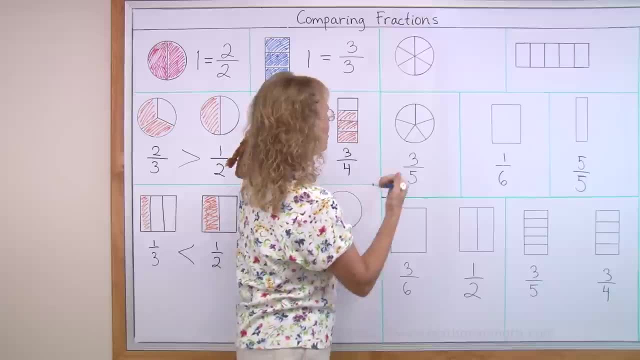 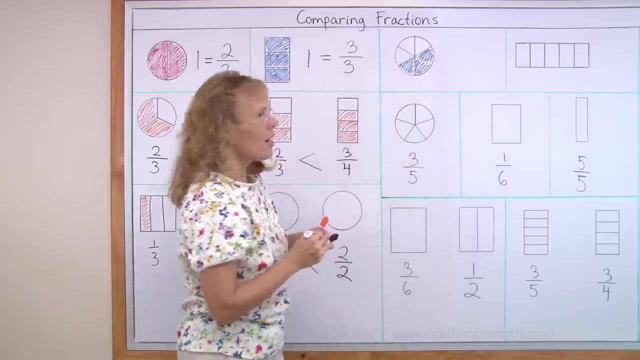 One sixth, And let's say that I color a few. Oh, Matti wants to color again. Well, soon, Matti, Soon Matti, I'll color. this time I colored three of those sixths, So I write a fraction. 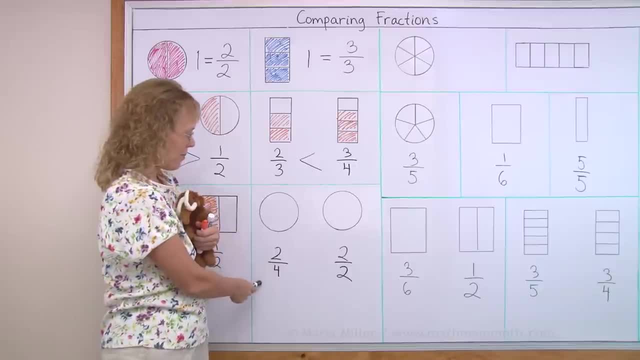 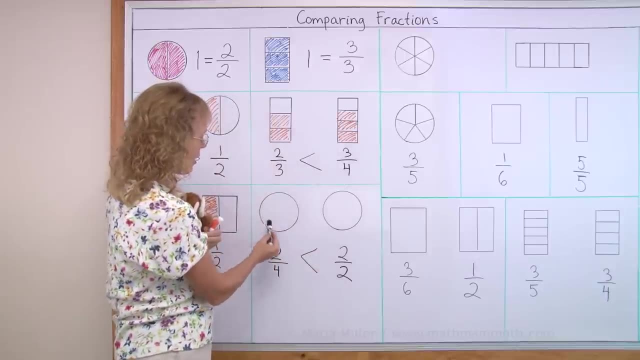 pie Here. I won't color the whole pie, So I can save some time and just tell that this is the greater fraction. right, That's the whole pie. This would be, you know, if I divide it into fourths and then color two. Let's go on. 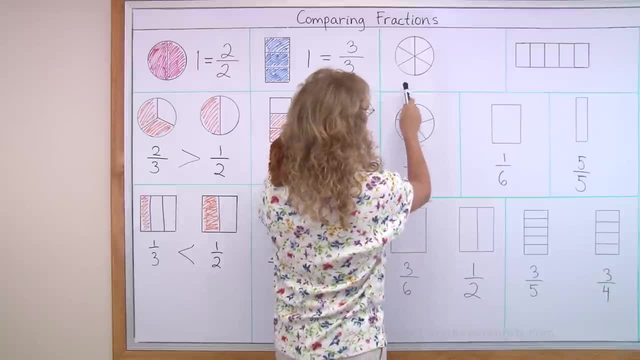 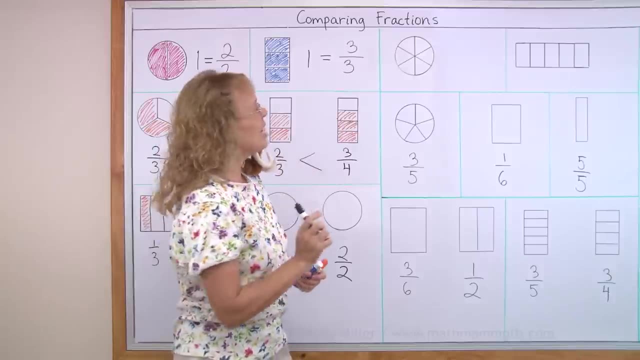 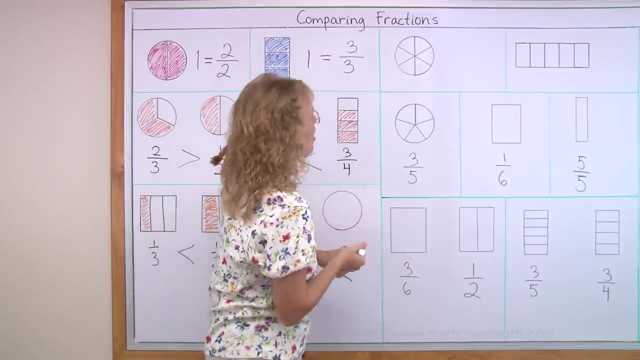 Over here. Well, Matthew, go back. How many parts is this pie divided into Six parts? So each part is a sixth, one. sixth, And let's say that I color a few. Oh, Matthew wants to color again. Well, soon, Matthew. 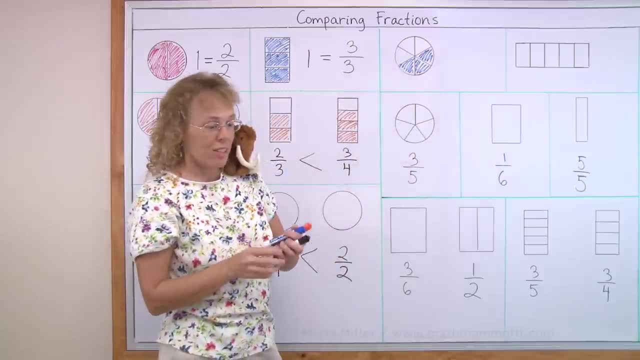 soon, Matthew, I'll color this. I colored three of those sixths, So I write a fraction Three, then I divvy them Right, so now I have six. I dip them Правильно. How do you do Atari versus proof? Well, nossa, put one in the opposite direction, thereacs. 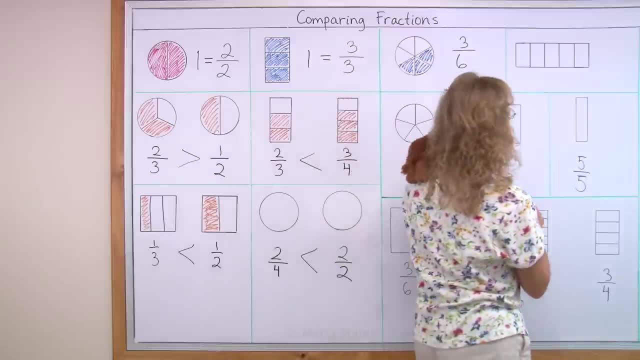 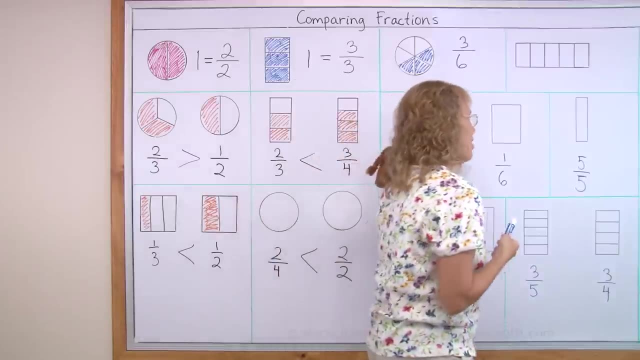 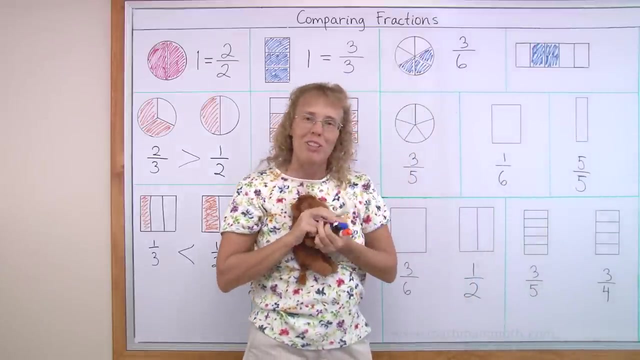 And then over here it's divided into five parts, so each part is a fifth. And Matti, yeah, I'll let you colour this time. So what fraction is coloured by Matti? Two parts are coloured, five in total. 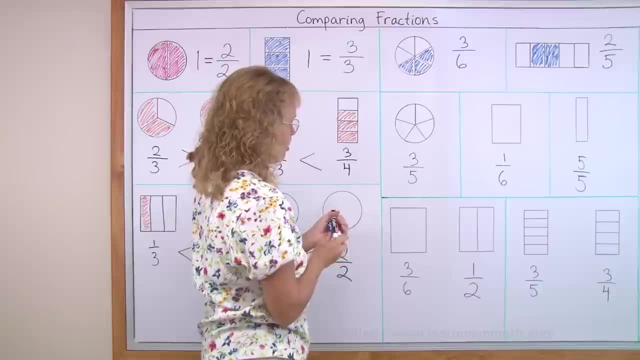 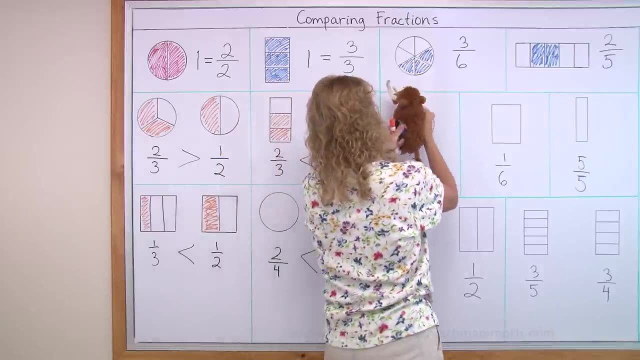 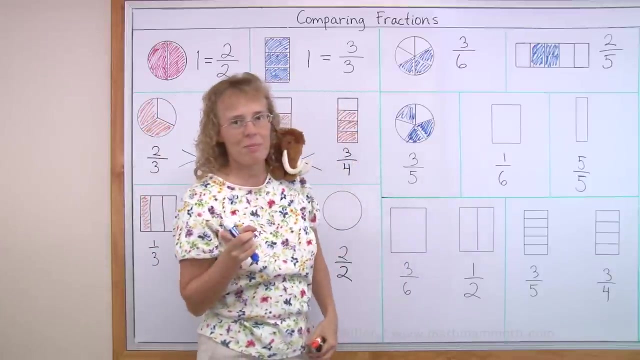 Two fifths. Oh, here's some more colouring to do. Matti can come down again. Colour this one. Three fifths. Fractions are so much fun because you get to colour so much. Now it's my turn. What fraction is this? 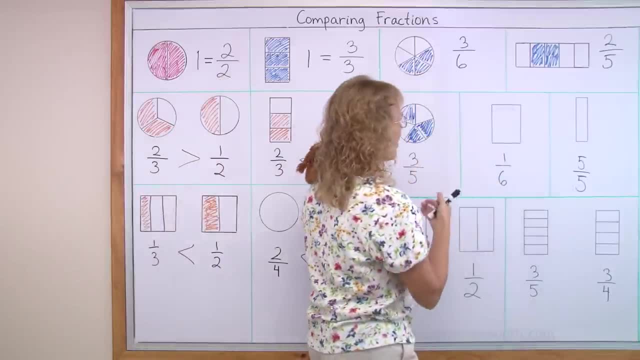 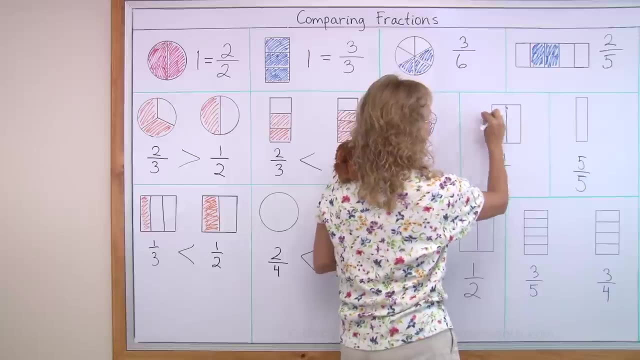 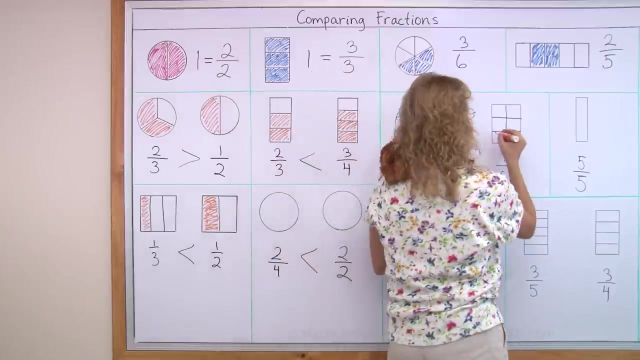 One, sixth. So I need to first divide this thing into six parts, which, let's say, I first divide it into two parts, like that, And then I go this ways: two lines like that, And then colour one Over here. five, fifths. 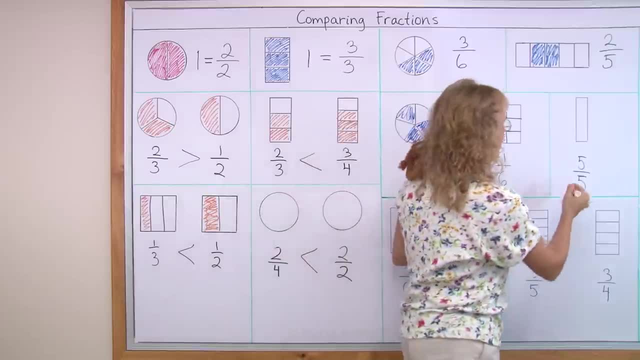 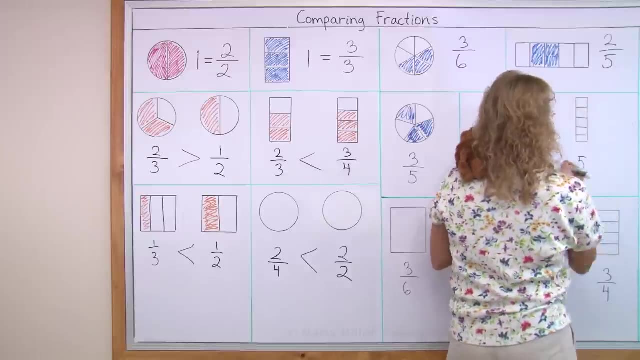 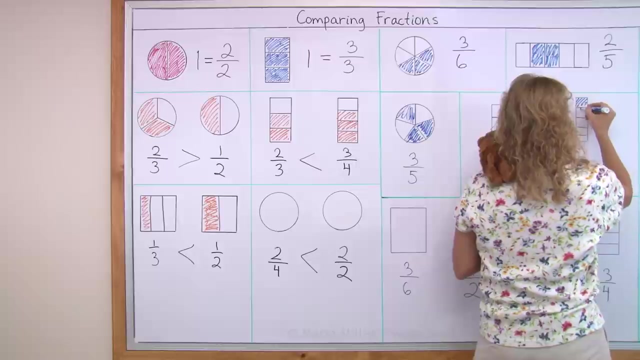 Actually, that's going to be the whole rectangle, One whole, But I need to still divide it into five parts and colour five. so let's try. Oops, those didn't end up being equal parts. Okay, they shouldn't be, So I didn't do a perfect job of dividing it, but I'll colour the whole thing anyway. 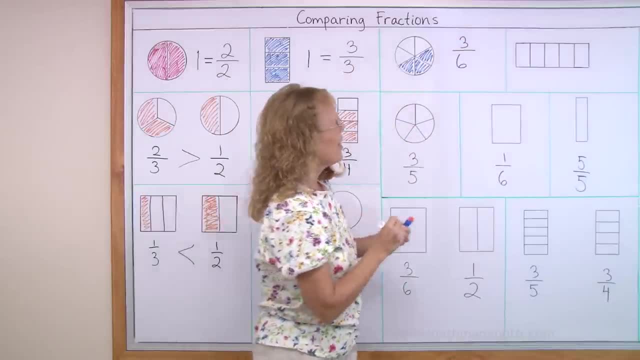 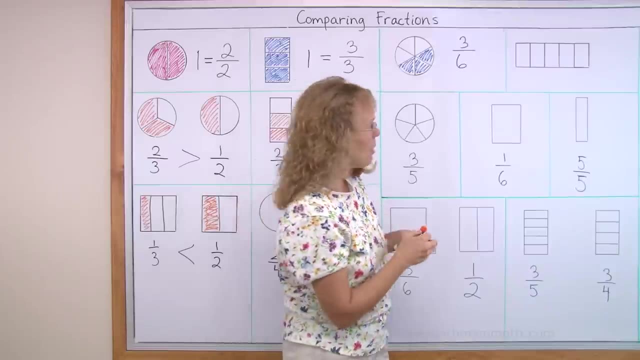 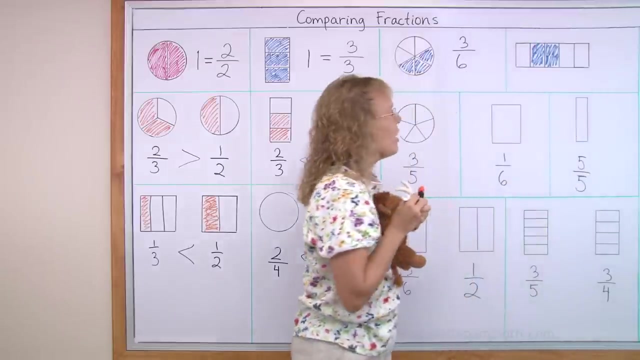 Three, Three, sixths, And then over here it's divided into five parts, So each part is a fifth. And Matti, yeah, I'll let you color this time, OK, OK. So what fraction is colored by Matti? 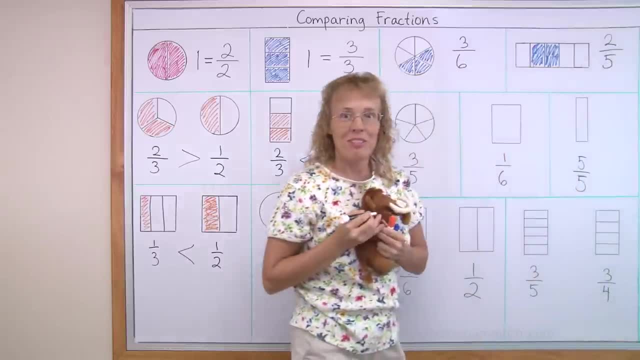 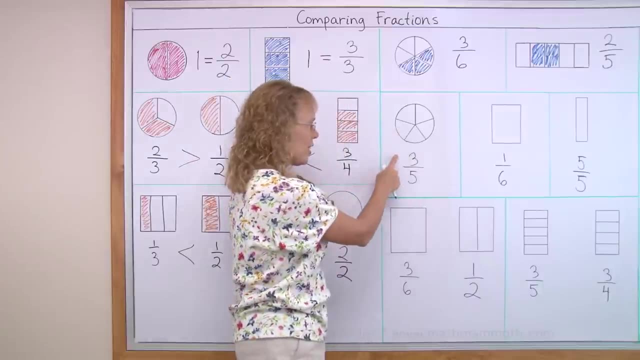 Two parts are colored, Five in total, Two fifths. Oh, here's some more coloring to do. Matti Calm down again. OK, Color this one. Three fifths. Fractions are so much fun because you get to color so much. 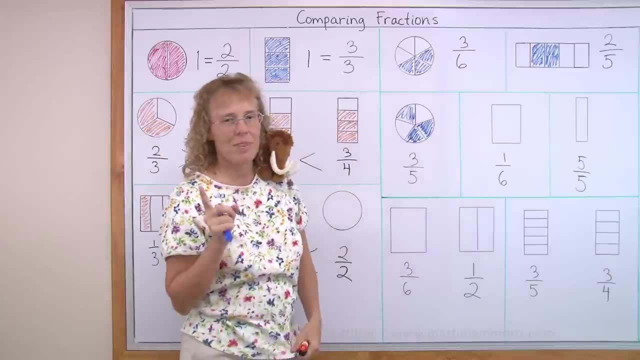 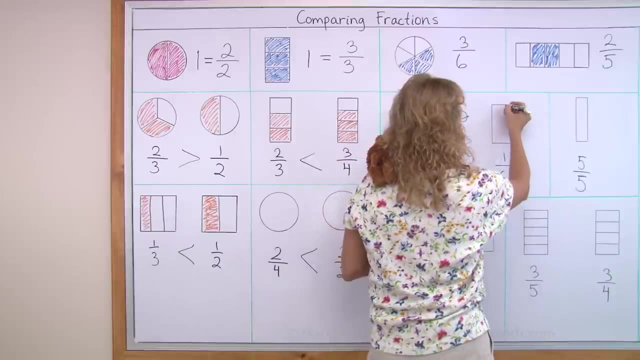 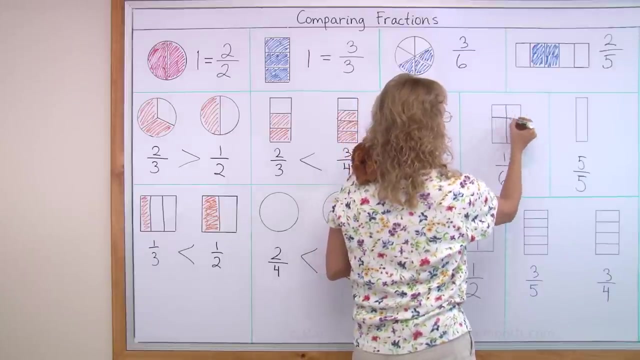 Now it's my turn. What fraction is this? One sixth. So I need to first divide this thing into six parts, which let's say, I first divide it into two parts, like that, And then I go this ways, two lines like that: 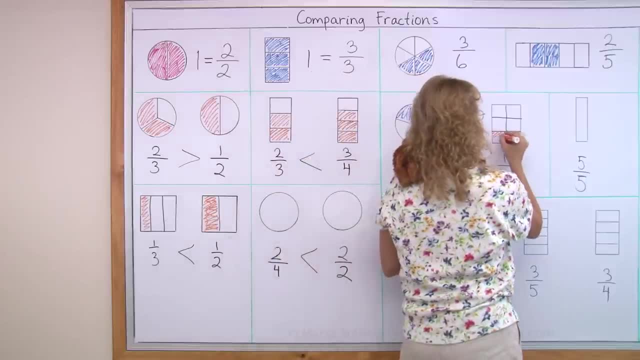 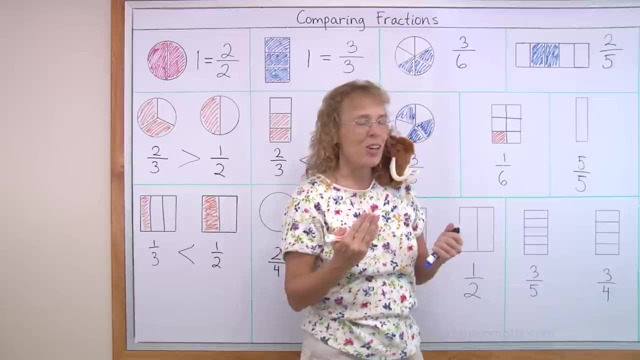 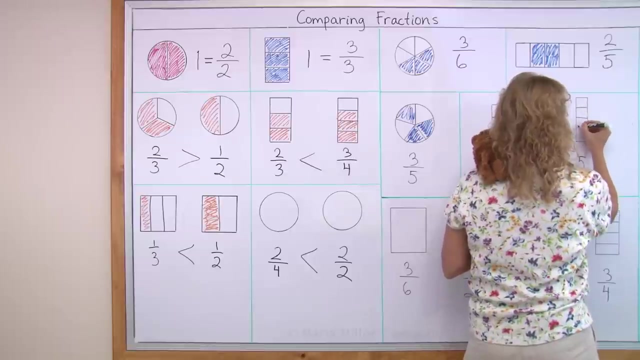 OK, And then color one Over here: five, fifths. Actually, that's going to be the whole rectangle, one whole, But I need to still divide it into five parts and color five. So let's try. Oops, those didn't end up being equal parts. 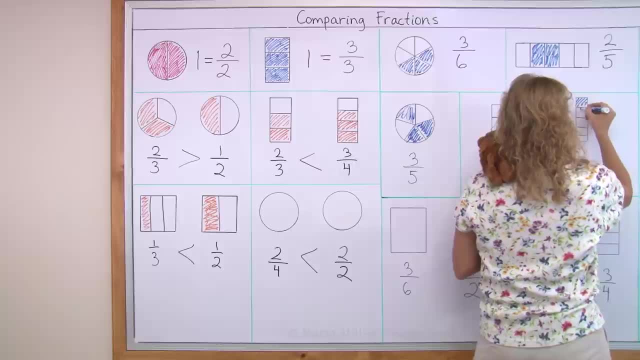 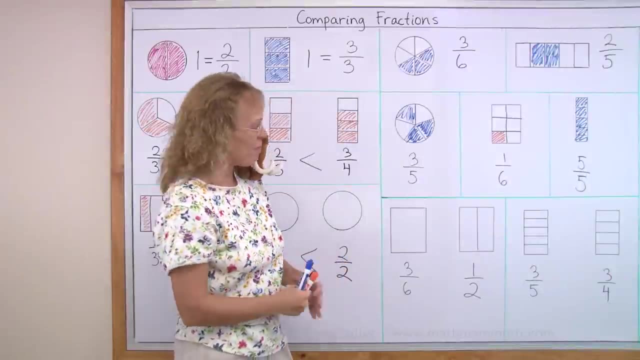 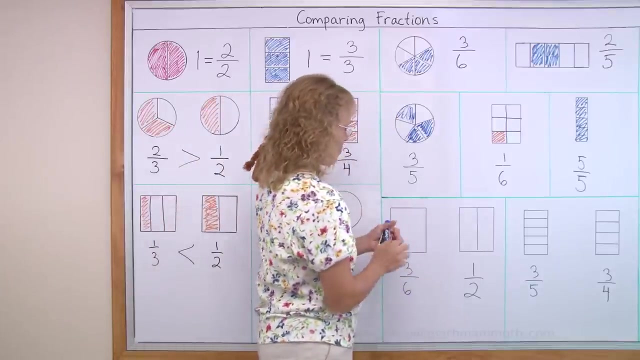 OK, they shouldn't be, So I didn't do a perfect job of dividing it, But I'll color the whole thing anyway. Lastly, we get to compare again which fraction is greater? Want to guess Three sixths and one half? 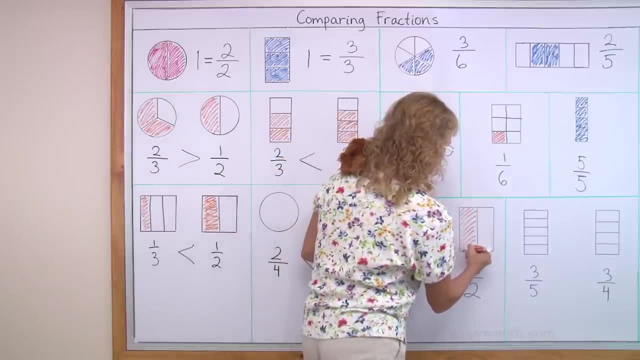 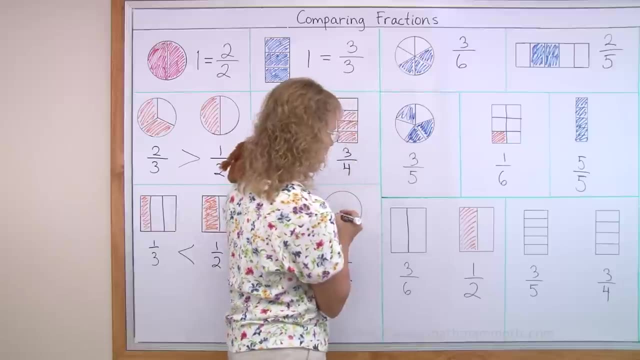 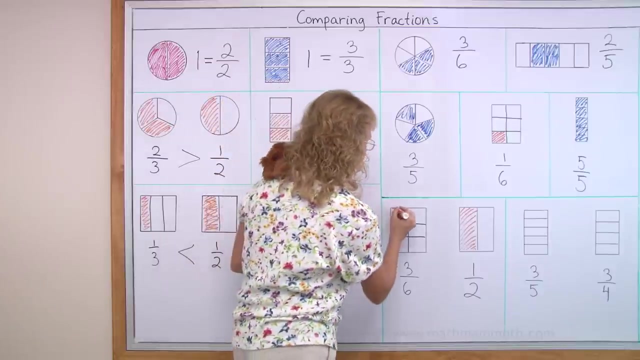 OK, the one half is already there, Just color it in. And now three sixths. First of all, I will divide this in half and then, with two lines like that, Now I will color three sixths. I'll color these three. 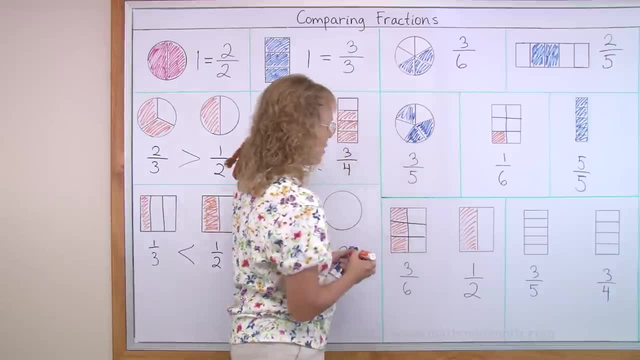 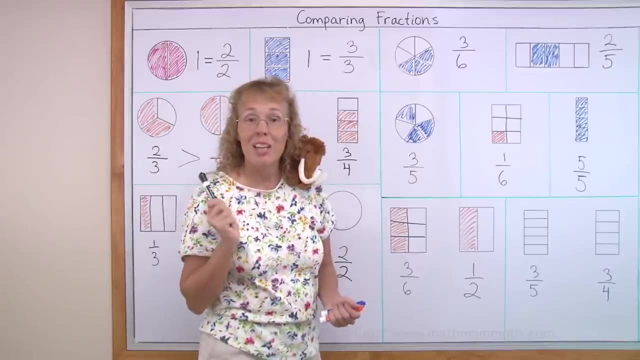 Of course you can color any Three pieces, But for comparing this makes it easier. Can you see which one is more? You know? this time they are equal. right, It's the same amount of chocolate bar to eat this way.